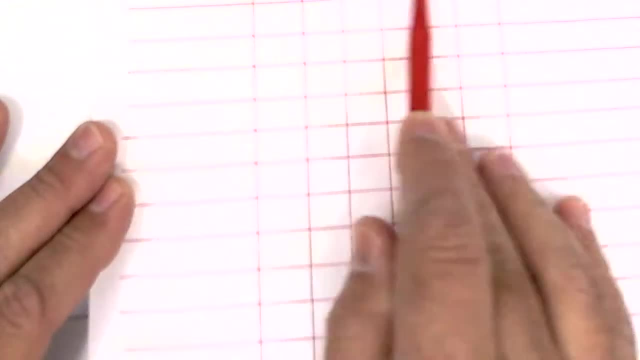 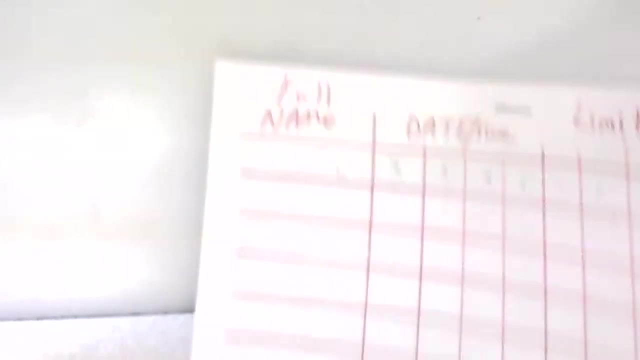 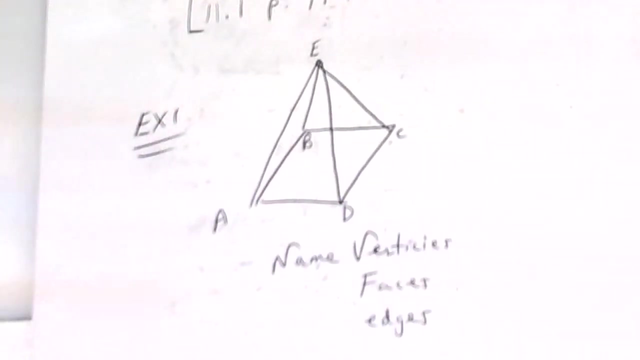 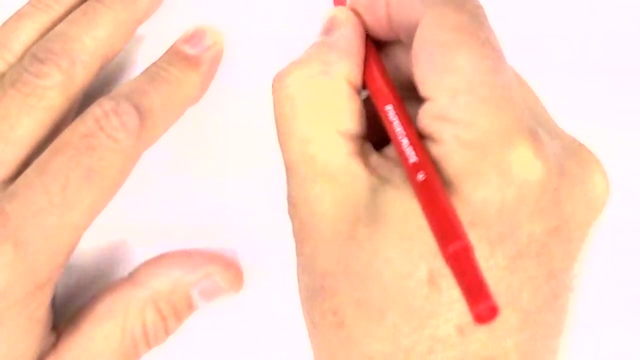 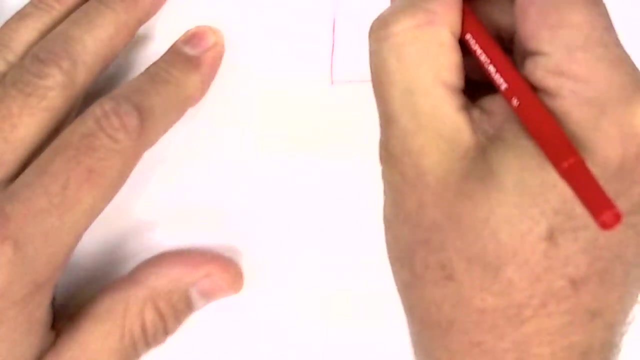 So hopefully six is enough. If it's not enough, maybe they can go to a different period or before class. Okay, let's go. Okay, let's talk about today's lesson. Yesterday we talked about polyhedrons. If you take a square and put a dot at about 12 o'clock and connect these dots, 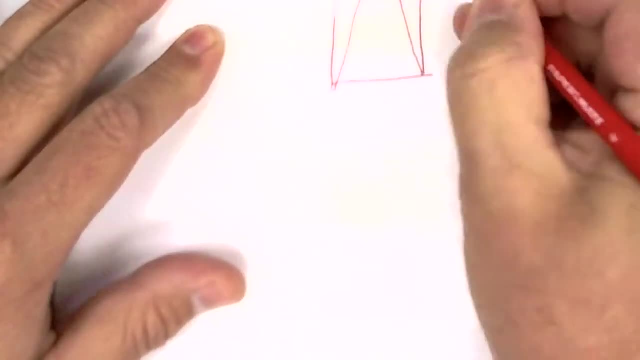 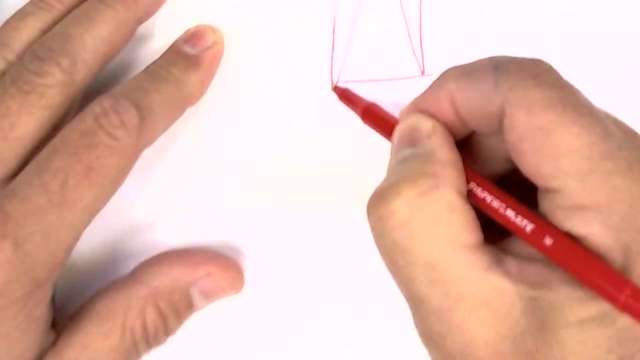 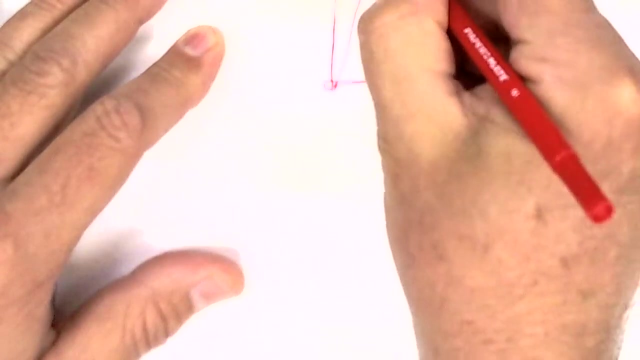 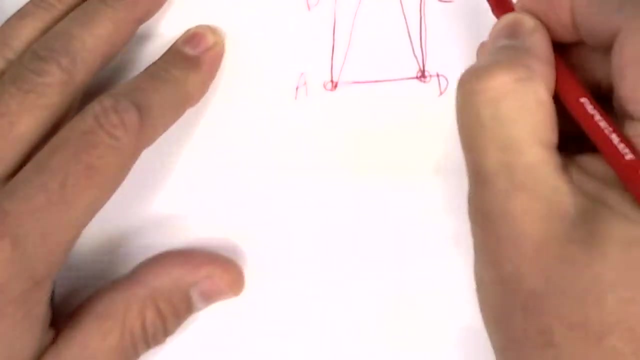 you have a square pyramid. A pyramid comes to a point. Anything that comes to a point is called a pyramid. Since the base is a square, it's called a square pyramid. These points- one, two, three, four, five- are called vertices. So the vertices are A, B, C, D. 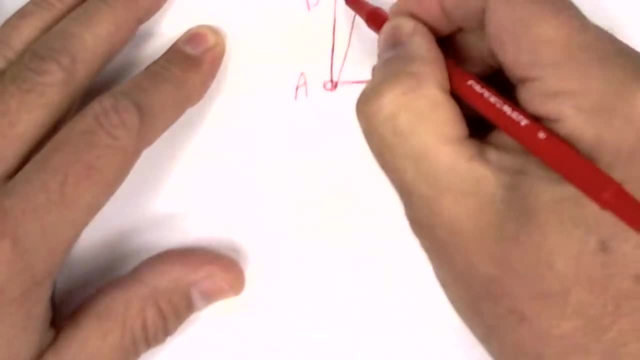 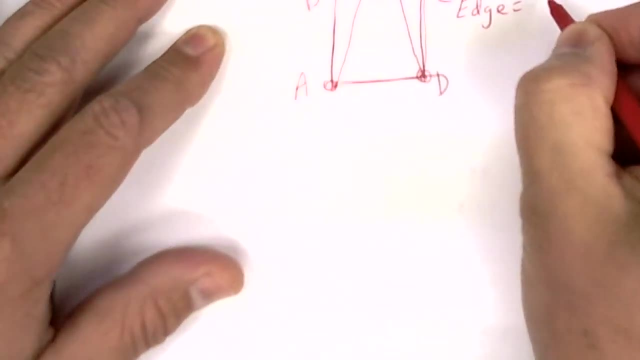 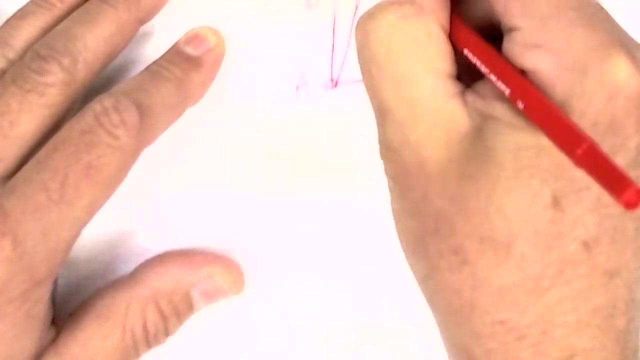 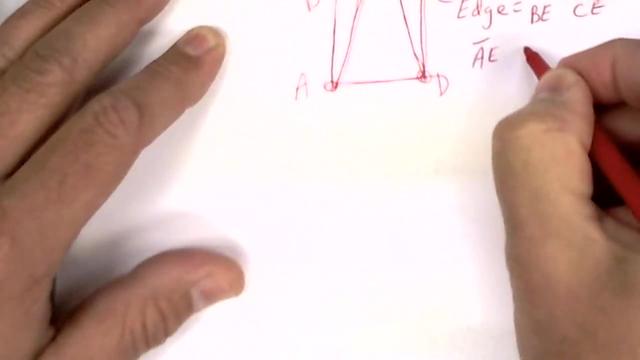 And there's five of them. This side, right here, is an edge. So you would say segment B- E, Segment C: E is edge, Segment A: E is an edge and segment D-E is an edge. Those are the edges. 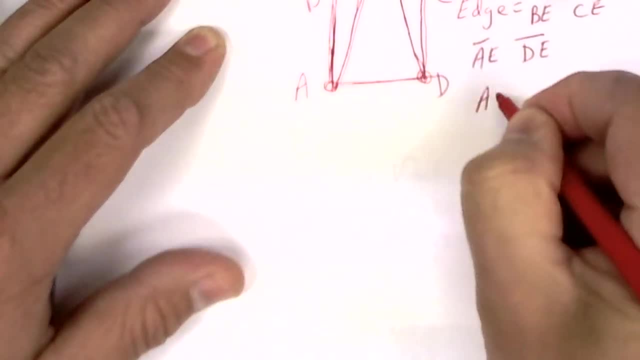 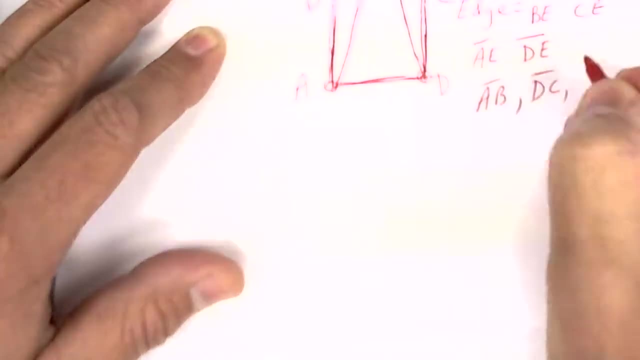 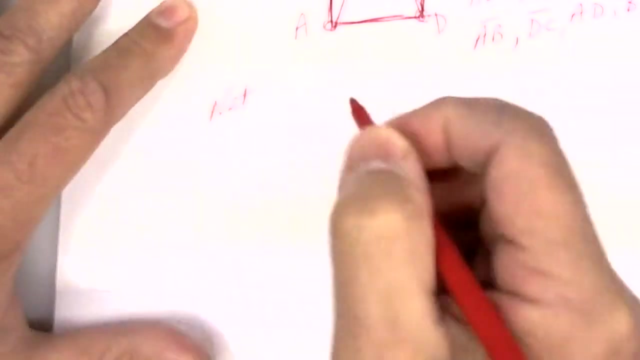 And then you've got some down here: A-B, D-C, A-D and B-C. Those are all edges, The faces. if I open this up and do something called a net, like using a can opener to cut the seams, it would look like this: 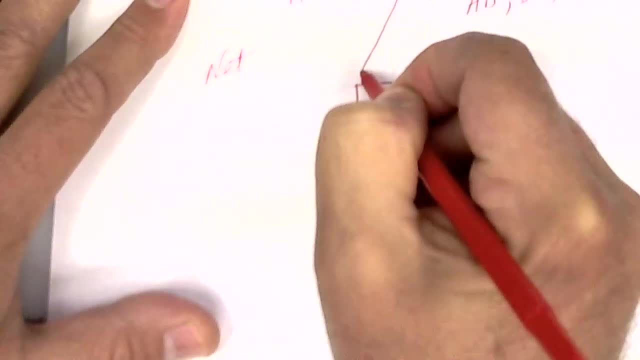 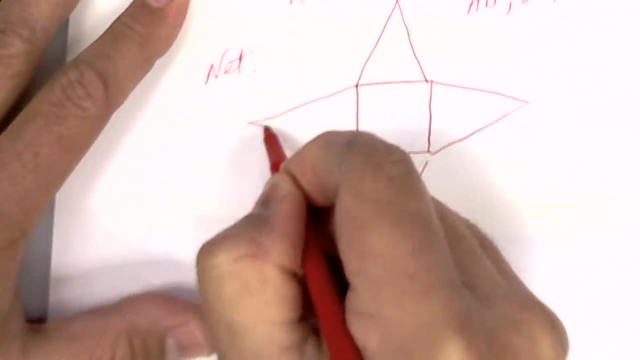 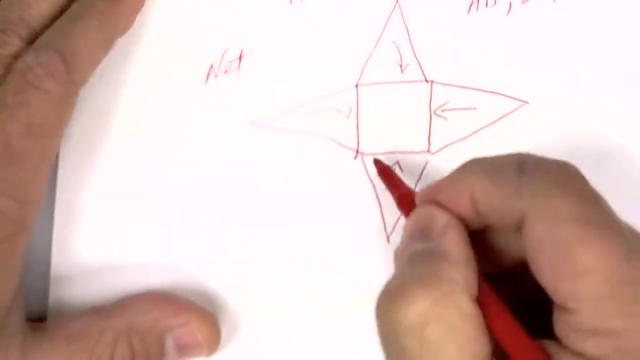 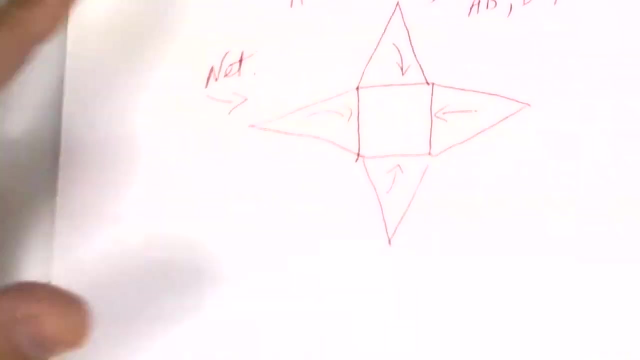 You'd have the base, a triangle here, a triangle here, here and here, And if you fold this up, you end up with the diagram. So this is called the net When you use a can opener on it. In any event, what's going to happen at this point is: 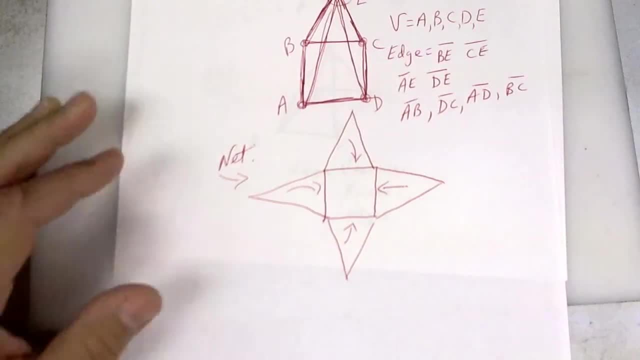 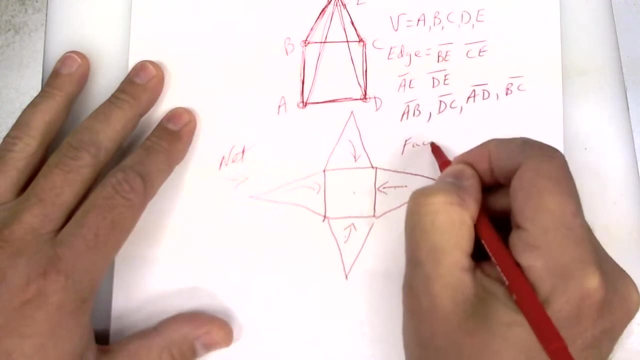 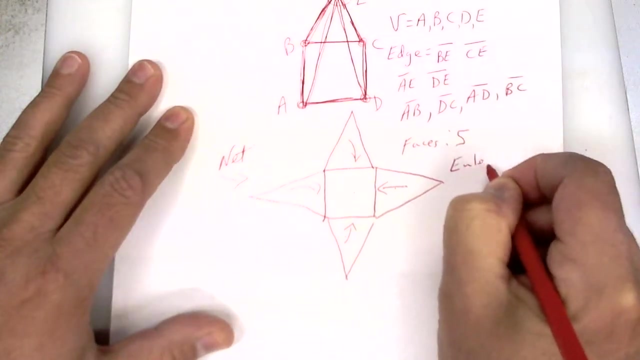 you've got to get the faces. So the faces would be all of these triangles, which is 4 plus the square, So the faces of the polyhedron on this example is 5.. Euler has a formula: F plus V, Faces plus vertices. 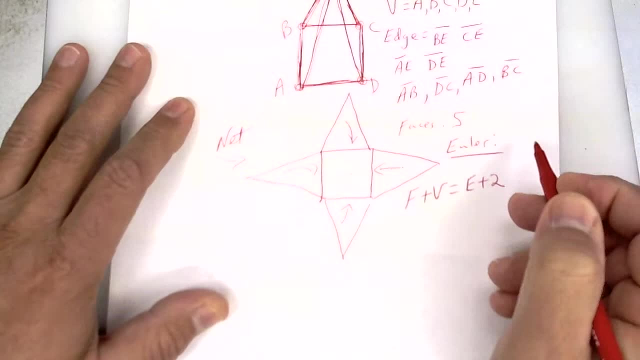 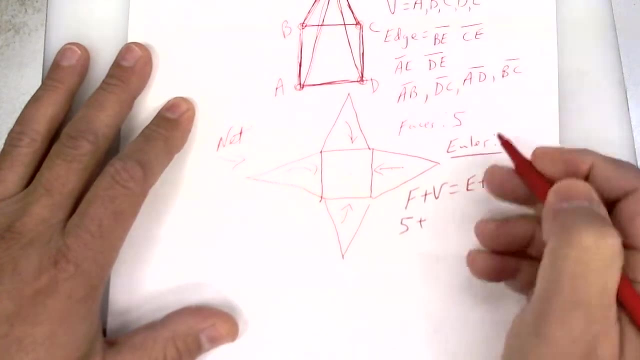 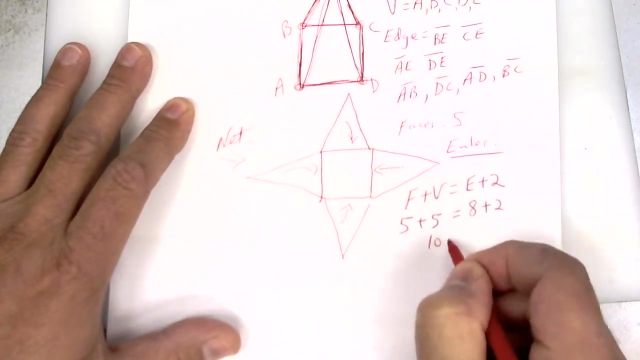 is equal to edges plus 2.. And let's check and see if that works Well. the faces is 5.. The vertices is 5.. Remember the points? The edges are 8.. And 5 plus 5 is equal to 8 plus 2.. 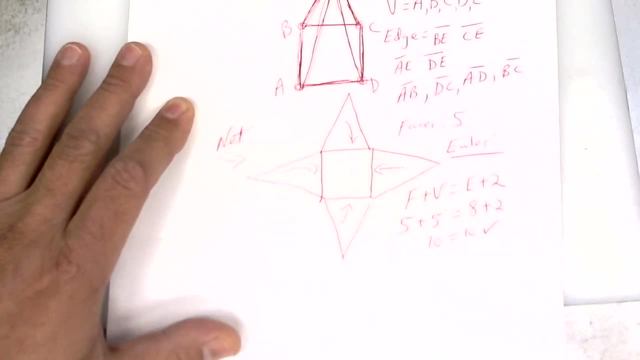 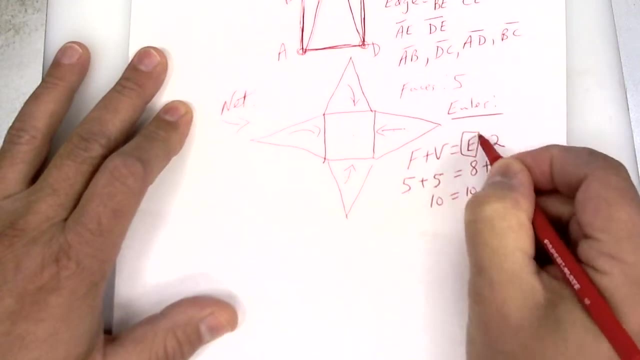 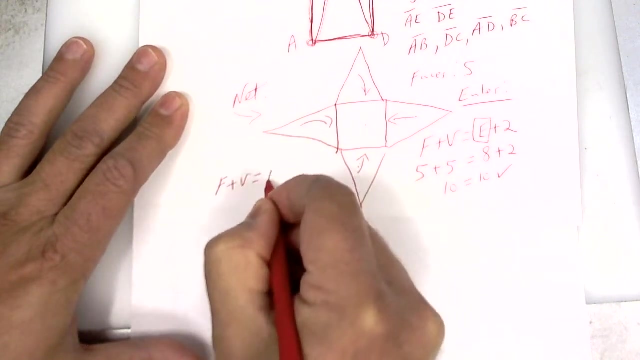 So Euler's rule works here and there it is. let's say, they did not give you the edges just for the sake of it, but they give you the faces and vertices. so faces plus vertices equals edges, which is what we're looking for. plus 2. let's just say: they didn't give you how many edges. well, you have. 5 plus 5 is equal to X plus 2. 10 is equal to X plus 2. subtract 2 and you get X equals 8. so there are 8 edges, and that's how you can use his rule or law or formula as well. we're going to do. 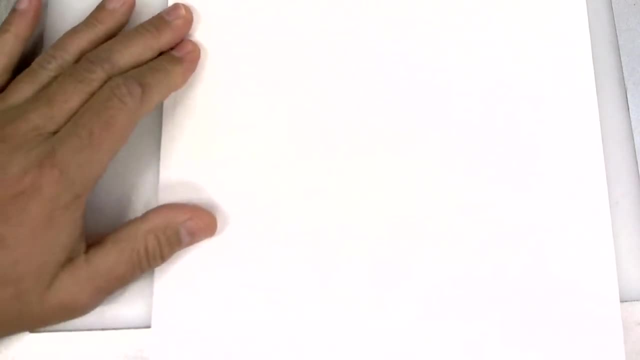 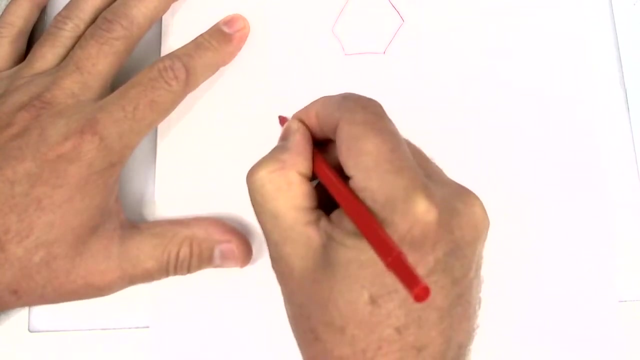 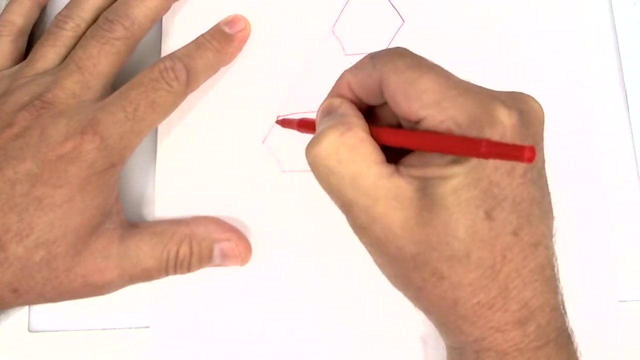 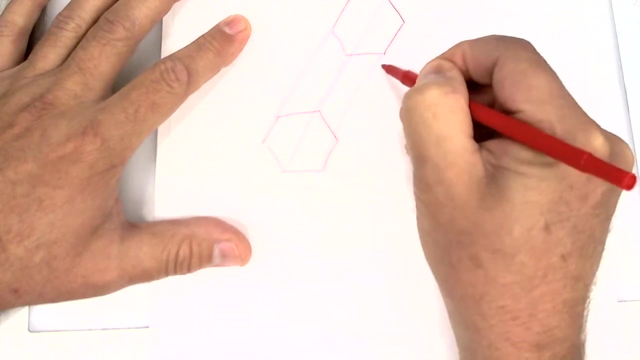 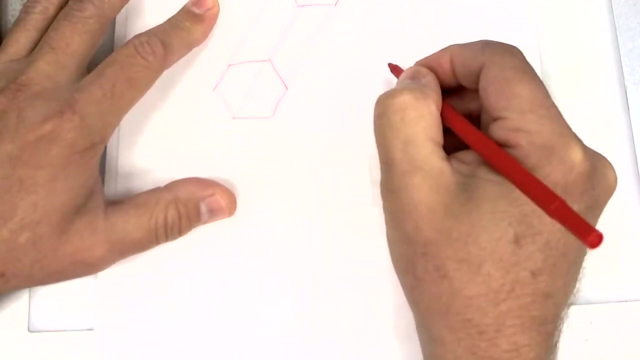 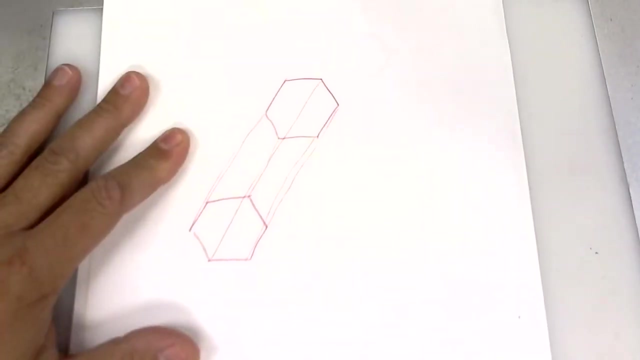 something called a hexagonal prism. you draw a hexagon, six-sided figure, you draw another hexagon and then you connect the vertices as best you can and you have a hexagonal prism. if you open this up with a can opener, it looks like this: if you open this up with a can opener, 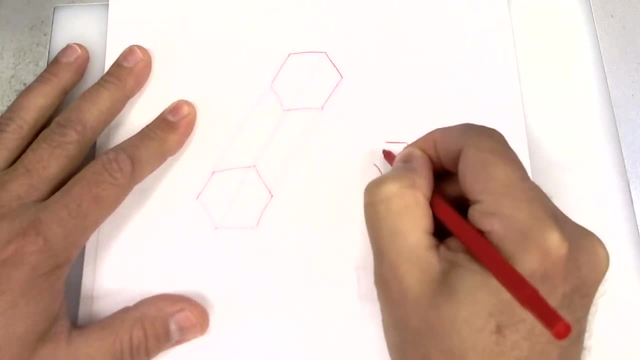 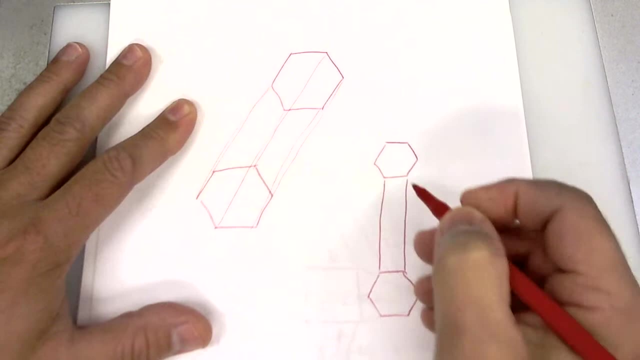 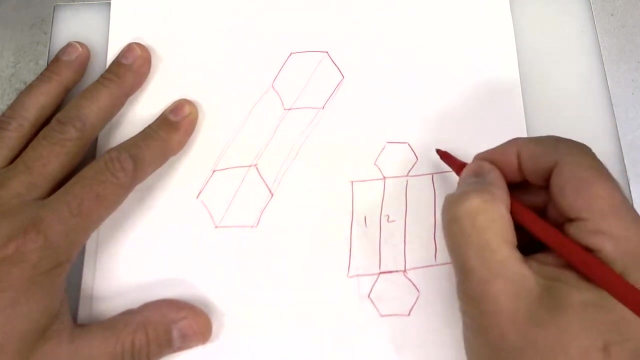 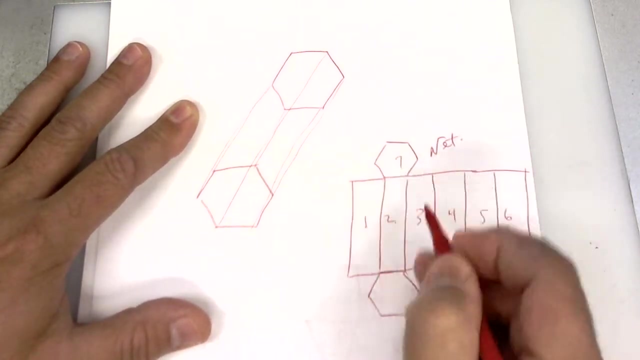 it would look like this: a hexagon, a rectangle and another hexagon, and then you have six sides. so you're gonna have six rectangles: one, two, three, four, five, six rectangles. and there it is, and that's called a net. these are your faces: four, five, six, seven, eight.